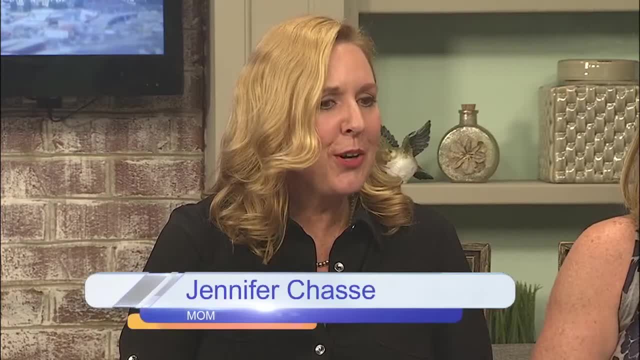 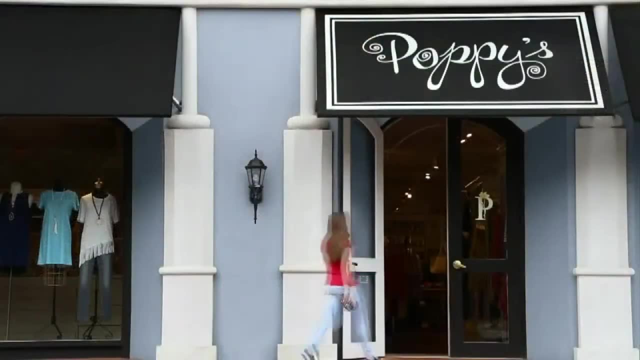 They're not charging, but you're giving them a debit card that's controlled from a free app for parents. Okay, So I can put money into their account and I can control how they spend it Really. Okay, So I can do things like control what types of stores they shop at, or even which stores they shop at. 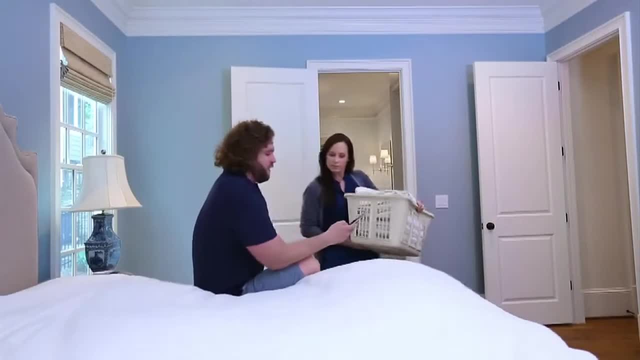 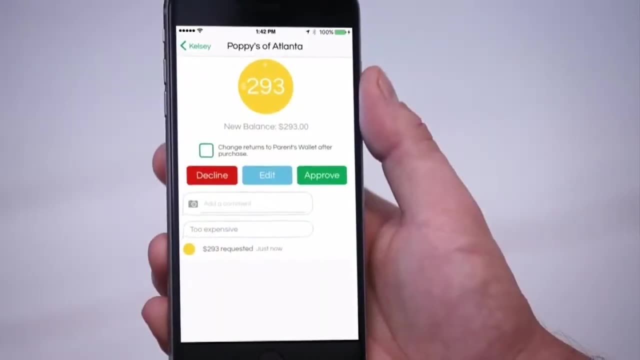 Okay, I can control how much they can spend. So I'm using it as a tool to try to teach my children budgeting. You know, a few months ago we started giving our kids allowance at the beginning of the month, hoping that they would learn how to budget monthly. Right, But you know I have a son that will spend all his money on pizza in the first weekend. Okay, So this way you can actually put controls in line, saying you can only spend X amount of dollars this month, Right. 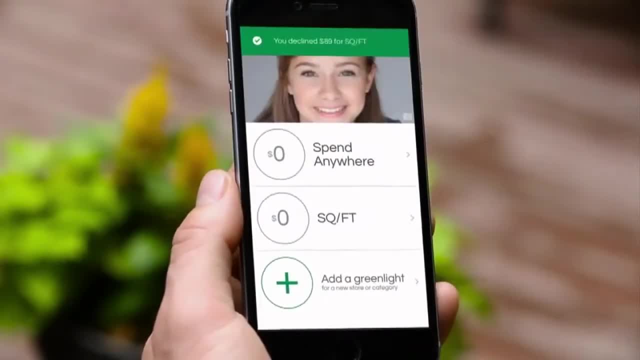 I feel like this is kind of a great way to show them wants versus needs, Exactly, Exactly. I mean you give them their budget and then they can decide: should I spend it on this? And then if they run out of money, they run out of money. 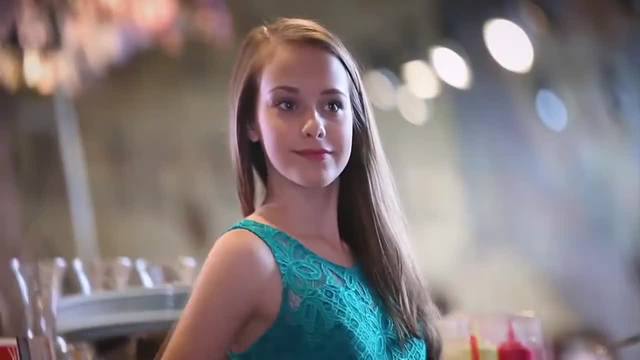 And what's really cool with the app and the control is that you get an instant notification on your phone. Okay, So when my kids were at Walmart buying baseball cards, I got an instant notification how much they spent. Right, They also can request more money from you. 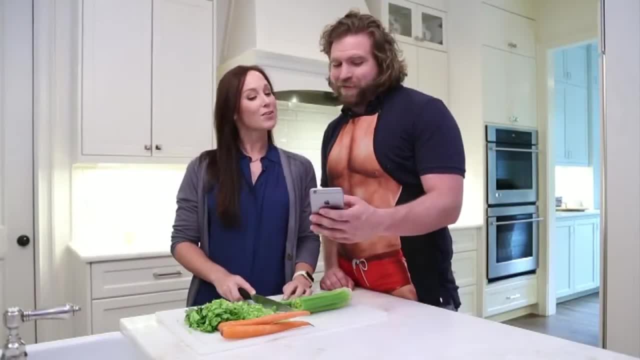 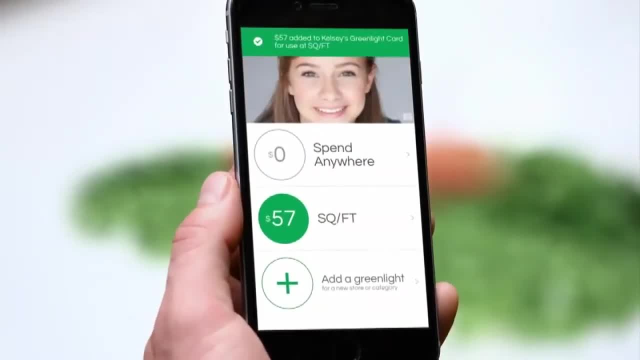 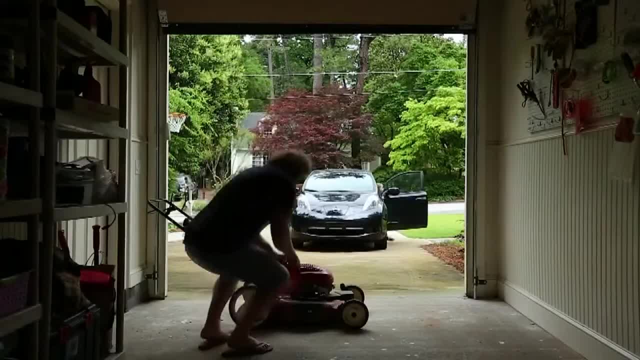 Okay, And they can even take a picture of the product that they want and send it to you and say, hey, can I get this? Here's how much it costs, Right, And it's instant. It goes straight to you, It's instant. 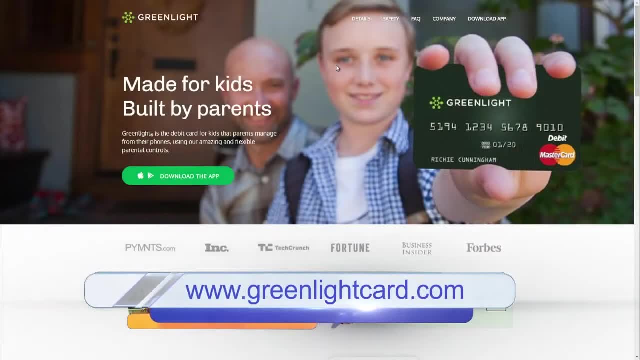 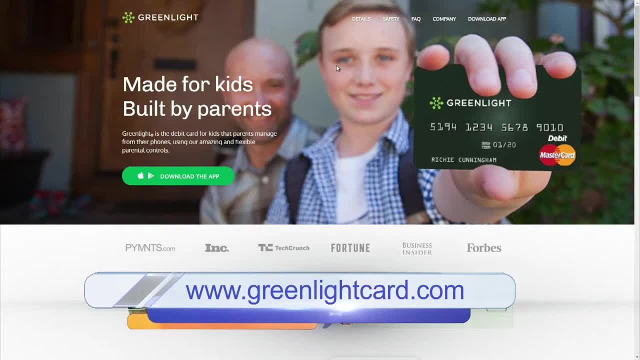 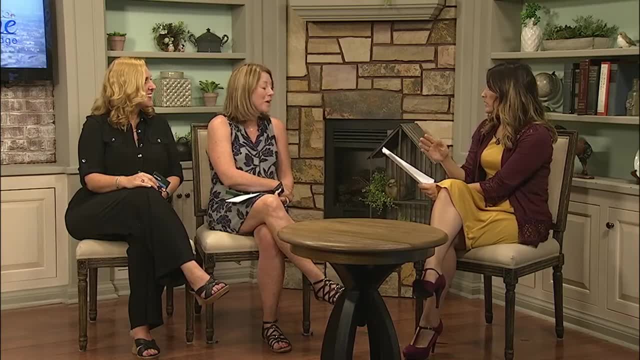 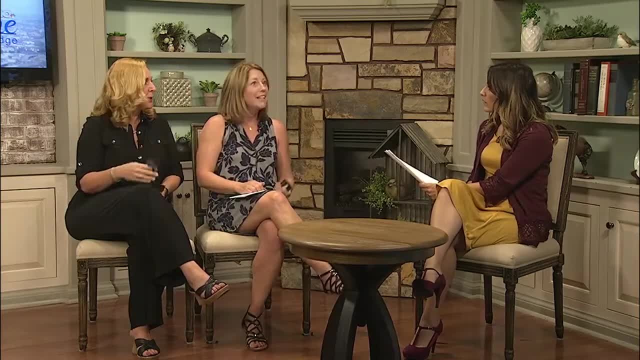 Yeah. Or you know, I can send my son shopping and say: find a pair of sneakers for $100. Right. And he can send me a picture saying: I really like this pair. It's $110.. Right, And I can instantly say sure.